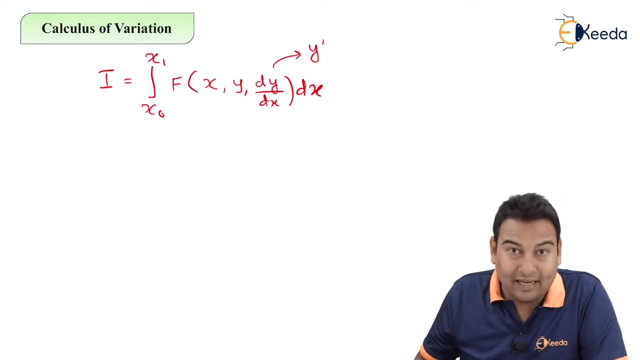 called maxima or minima, For finding that we do have Euler's equation. So let me write it down: the Euler equation and my aim is to get the value of y. This is my aim, this is the solution. y is equal to m. 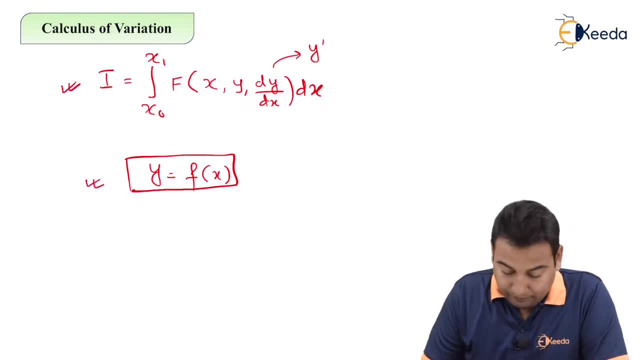 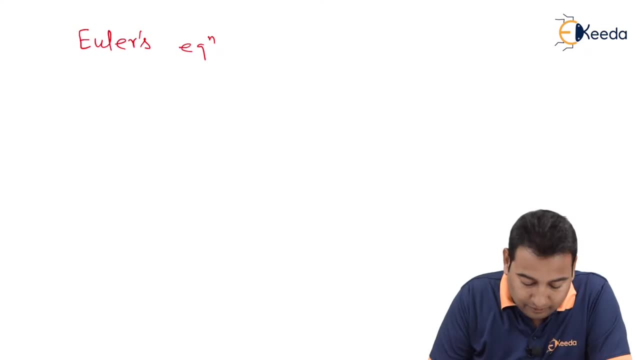 F of x. Problem is this and solution is this. Let me write it on the Euler's equation. That is Euler's equation First: is dou f upon dou y minus d, by dx of dou f upon dou y, dash equal to zero. This is: 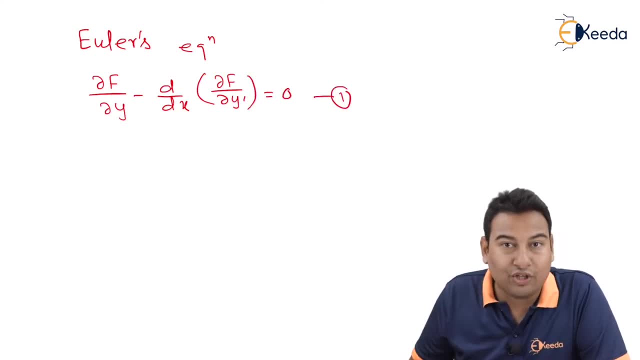 equation number one. We do have one more equation. This is the solution of the given integration, and that is number two- is dou f. So we have dou f upon dou x minus d by dx of f minus y dash, dou f upon dou y, dash equal to zero. 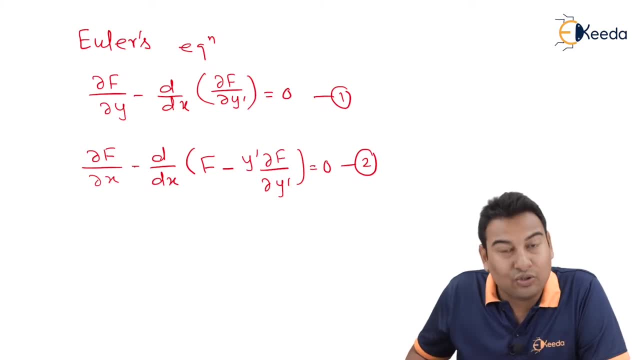 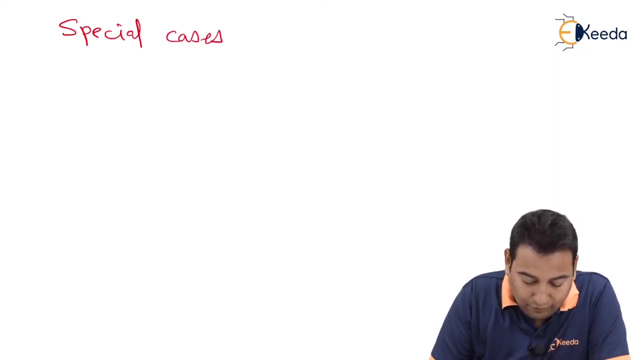 This is equation number two, Friends. these are the two solutions of this particular integration which is asked in the problem. Now, there are few special cases that you need to consider. There are three special cases. First is functional. F is called functional. It is not function. It is actually functional. is independent of y. 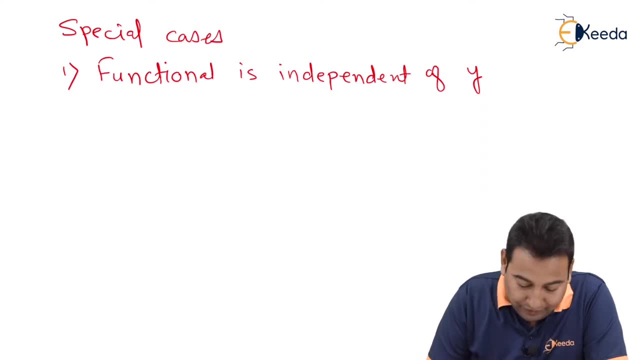 If functional is independent of y, what does this mean? If you differentiate that functional with respect to y, the answer is zero. This is for sure, because functional does not contains y. When you differentiate with respect to y, answer should be zero. 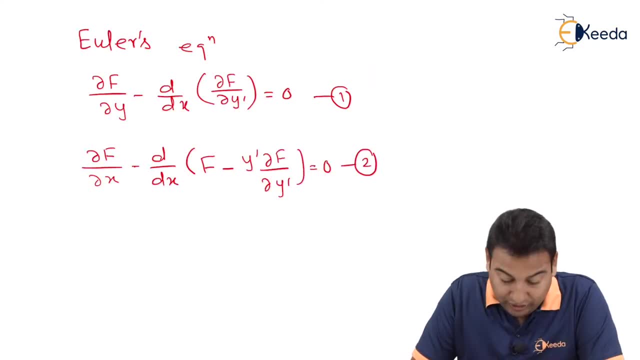 Now, friends, we have two options. Either you can choose equation number one or equation number two. Here we got dou f upon dou y, equal to zero. Let me check where exactly this term See here Dou f upon dou y, is. in equation number one, Let's substitute. 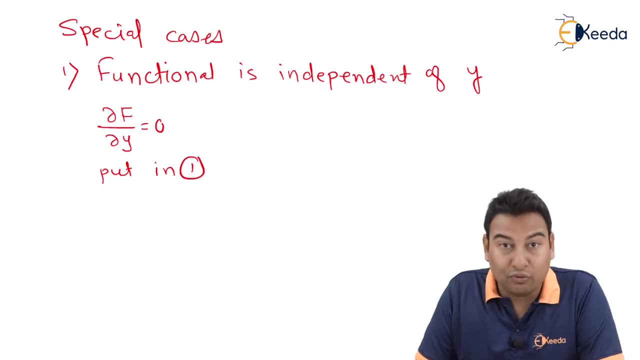 If I substitute dou f upon dou y, equal to zero, in equation number one, I will be left with the first term. dou f upon dou y will become zero. I will be left with Minus d by dx of dou f upon dou y dash, which is equal to zero. 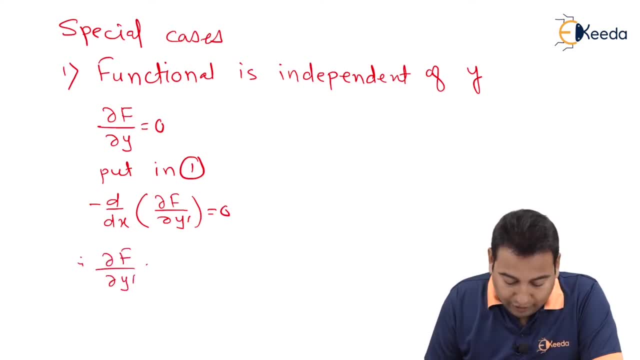 Therefore, dou f upon dou y dash, If this minus d by dx will go that side, that will become integration, and integration of zero is zero plus some constant which is equal to c. You need to remember: this minus d by dx will go that side and will become constant of integration c. 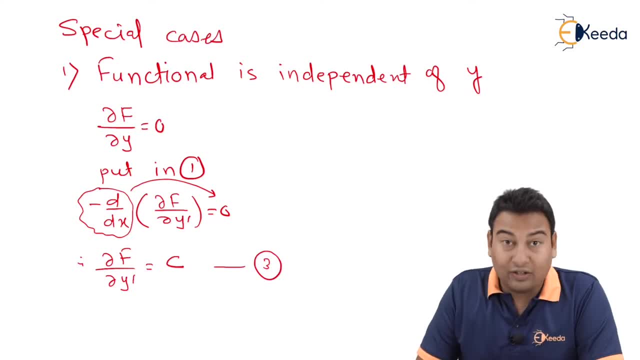 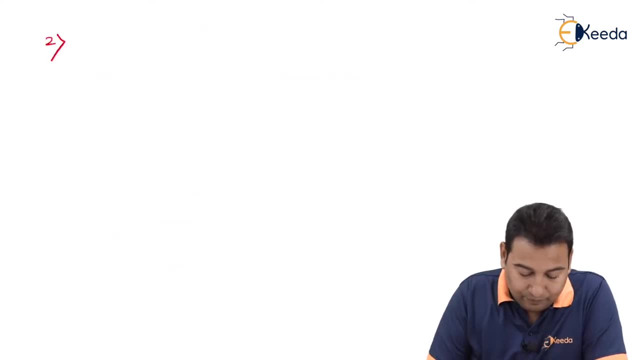 This is my equation number three. Now I got three equation: first, second and third. Let's move on. Now I'm going to consider the next case. Functional is independent of x. Friends, actually your original functional is in terms of x, y and y. dash, We're going to consider three cases. First it is independent of y, Then it is independent of x. 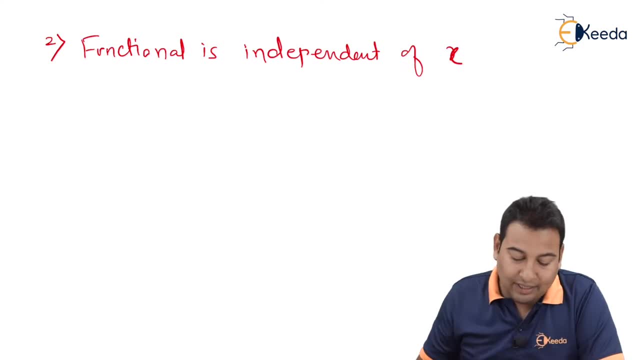 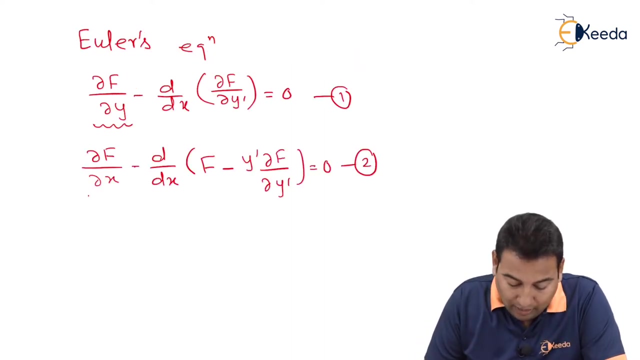 And finally, it is independent of y. dash Here. it is independent of x. Therefore, dou f upon dou x equal to zero. Let me check in which equation I'm getting dou f upon dou x. Check here, friends: Equation number one and two. In equation number two I'm getting this Dou f upon dou x equal to zero. Therefore, I'm going to put in equation number two: This term will be zero and I'll be left with this particular thing, That is, minus d by dx f. 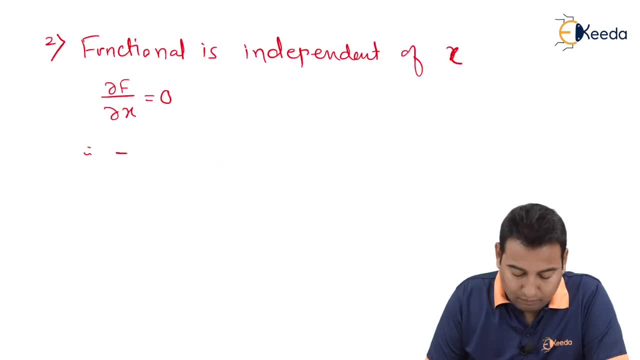 minus y dash dou, f upon dou y dash, equal to zero. Minus d by dx, f minus y dash dou, f upon dou y dash, equal to zero. Again the same repeated story. minus d by dx will go that side and will become c. Therefore it will be f minus y dash dou, f upon dou y dash, equal to c. This is the next equation. 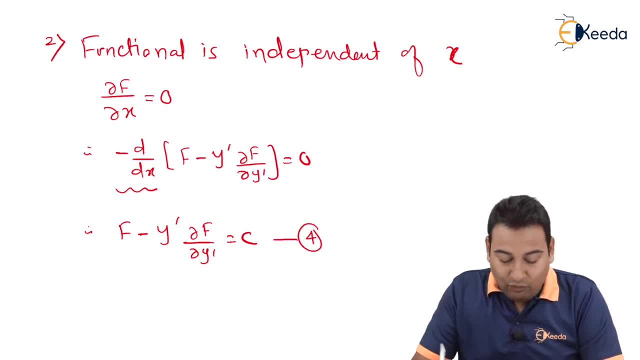 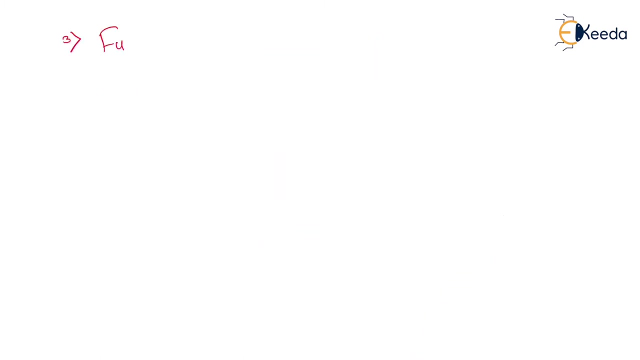 that is fourth one. there is one more case left. first we consider special case when a functional is independent of y. now we took functional is independent of x. what is last, functional is independent of y dash. let's consider that case. functional is independent of y dash, since it is. 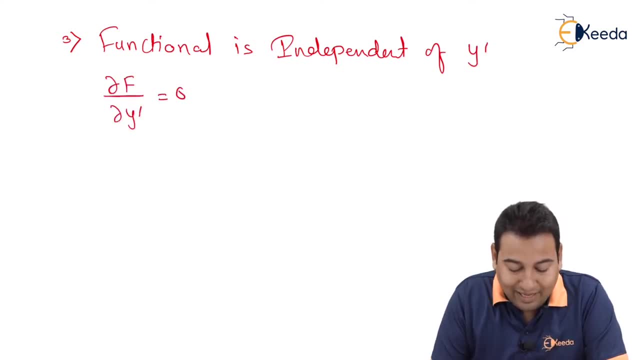 independent of y dash. if you differentiate with respect to y dash, the answer is zero. let me put this dou f upon dou y dash in one of the equation. let me check equation number one or two. where exactly i'm getting dou f upon dou y dash? now, friends, check in equation number one. 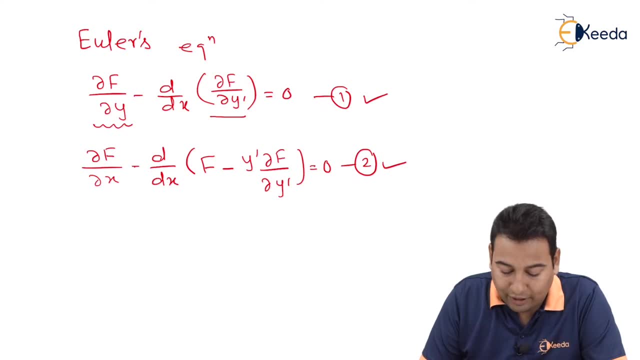 as well as two. in both equation we have dou f upon dou y dash. that means i can put in either of the equation. which equation you will choose? obviously equation number one, because if you put in equation number one i'll get the simple equation. therefore i'm going to substitute in equation number one. 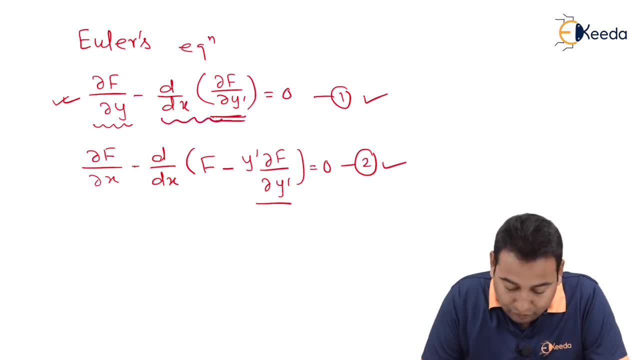 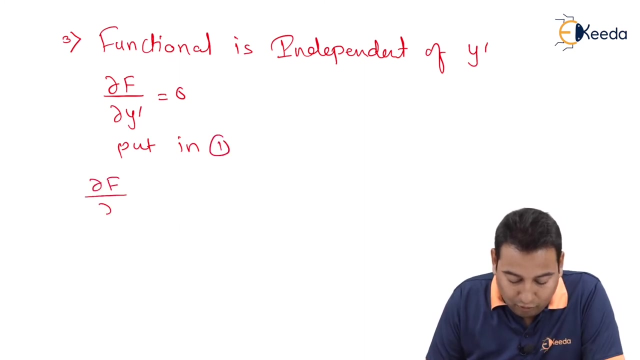 this particular term is zero. therefore, this will be zero and i will be left with dou f upon dou y equal to zero. let's put in equation number one. put in one dou f upon dou y, equal to zero. this is my fifth equation. friends, i got five equations, if you remember. 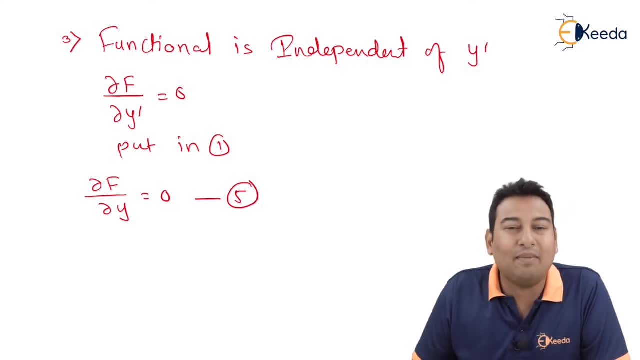 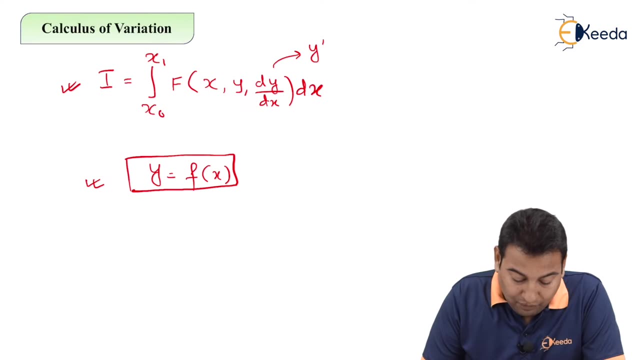 this equation you will get the simple equation. therefore, i'm going to substitute in equation number one- this is my equation- the problems you can easily manage, all the problems of calculus of variation. let's revise quickly. we started with. what is the aim of calculus of variation? we want. 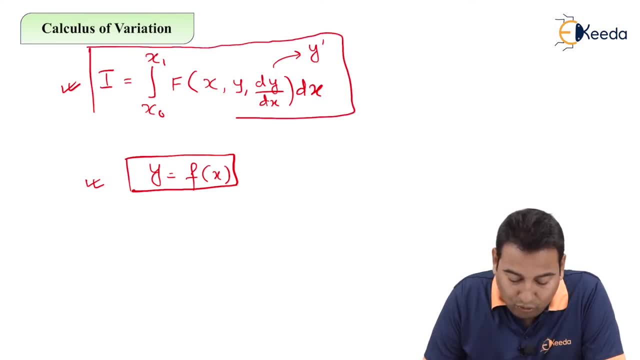 to evaluate this type of integration. or basically, i want to find the extremal point, or maximal or minimal point, or stationary points of this particular integration. that means basically my solution that i want is: y is equal to f of x. here this functional is integral of f of x, and i want to find the integral of f of x and i want to find the integral of f of x. 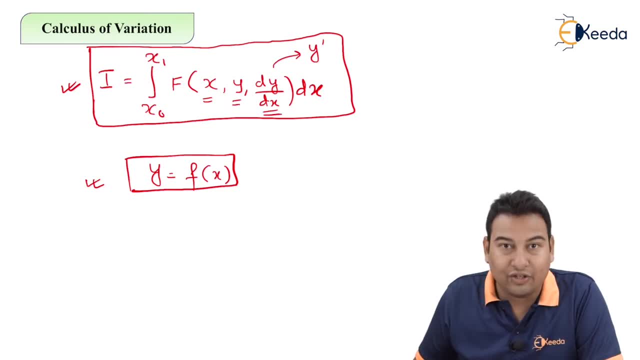 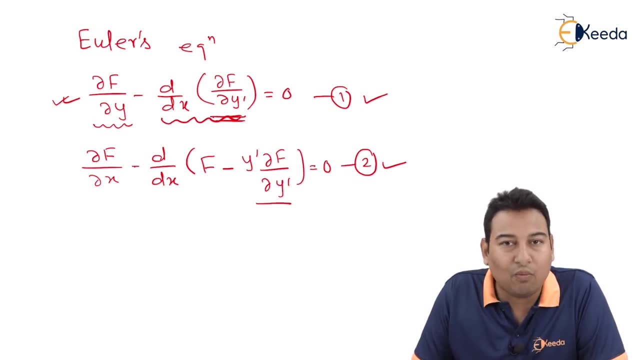 in terms of x, y or y dash- you need to remember this- to euler's equation. depending upon the situation, i'm going to use equation number one or equation number two, then there will be three special cases. once i'm going to consider, the functional is independent of y. therefore dou f. 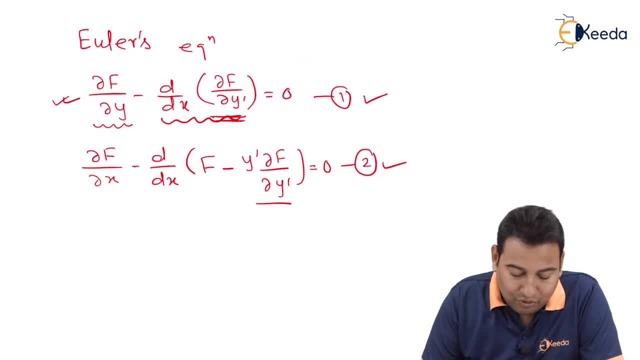 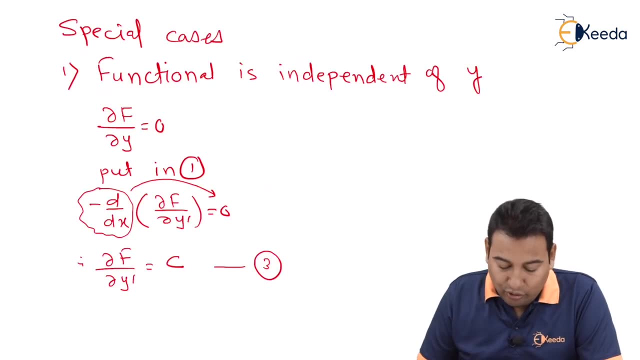 upon dou y equal to zero. and for that purpose i'll be substituting in equation number one, because dou f upon dou y is there in equation number one and through that i'm going to find the integral of f of x. i'm going to get dou f upon dou y, dash equal to c. next special case is: